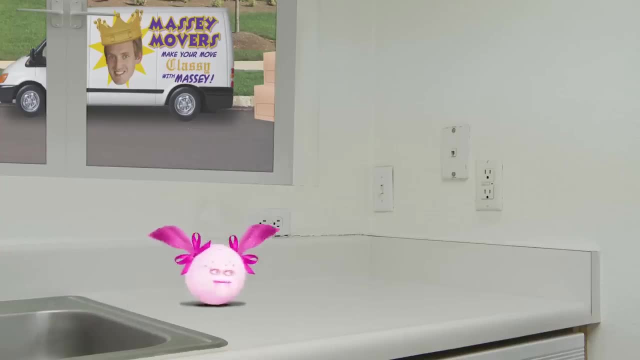 if you jiggled the Dr Pepper button, just right. Hey, where did everyone go? Are we playing hide-and-go-seek? That's like my favorite game. Well, my actual favorite game is Duck Tug Goose. 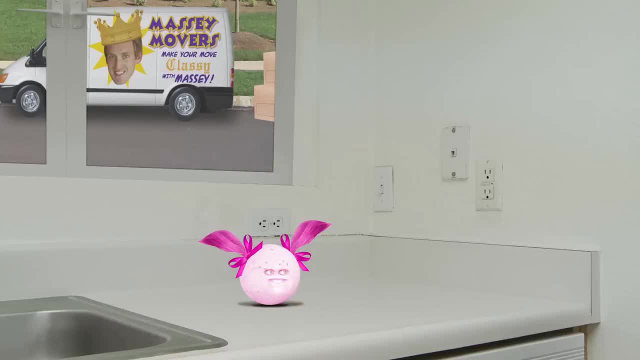 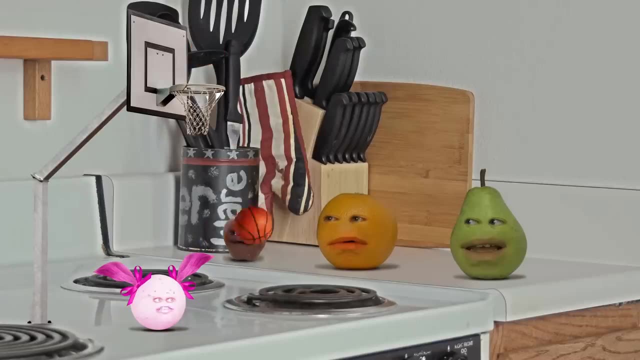 Okay, no, that's a lie, It's actually freeze tag, but I sometimes like tetherball. My grandma said that I was talking too much and that I should go over and meet our new neighbors and make some new friends, And so I came over here to say hi and to tell you that I have two ferrets and three gerbils. 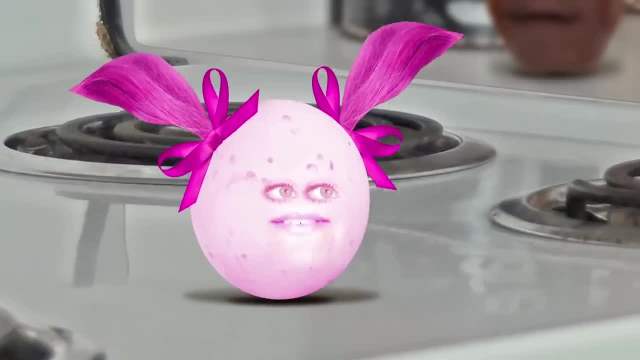 and the names of the ferrets are Furball and Muffin and the names of the gerbils are Snap, Crackle and Pop. And if you guys want to come over and see them sometimes you can. They're really nice, except Crackle bites sometimes. What are all your names? 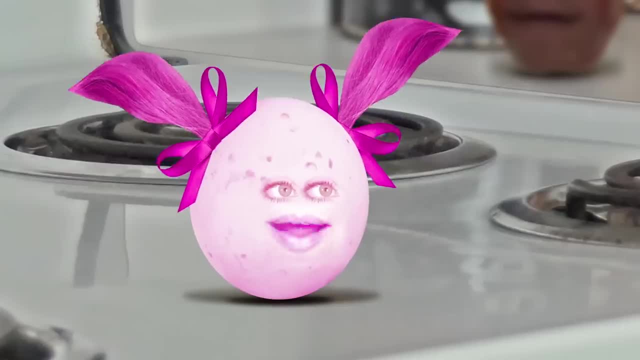 I'm Pear and this is Orange and this is I'm practicing to break the world record for the biggest bubblegum bubble ever blown. My brother says I'll never be able to do it, but my dad said I should go for it. 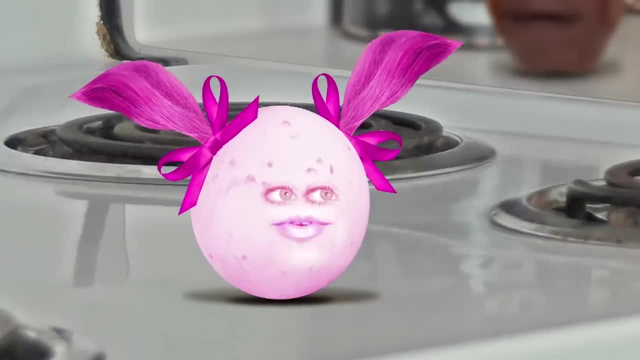 My mom said I should go for it too. I think they like it when I blow bubbles, because it means I can't talk while I'm doing it, but at the same time, they just might be supportive of my dreams. Hey, do you guys have grasshoppers here? We had grasshoppers at my old kitchen. 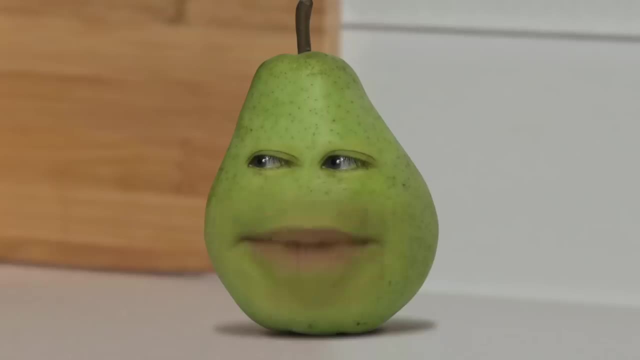 and I caught 34 of them in a jar and named them: Dave, Sammy, Mr Crickles, Roberto, Hey Bubblegum, Maybe you could blow a bubble for us right now. Good call, It'll keep her mouth occupied for a while. 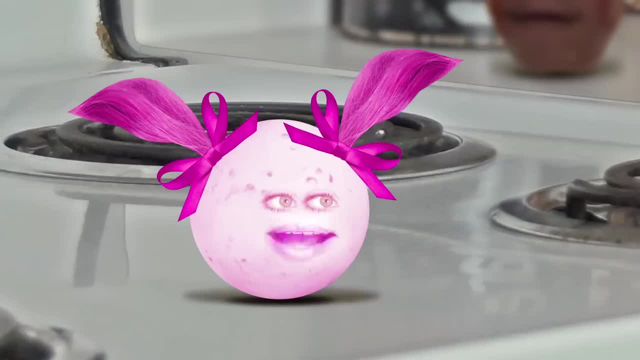 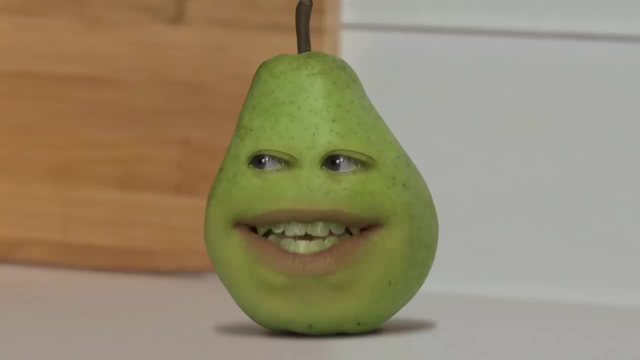 Blow a bubble for you guys. That's a really, really great idea, because I haven't practiced much today and I really should stick to my regimen if I want to break the world record someday. Ah, peace and quiet. Now back to horse. What does everybody have? I have an H. 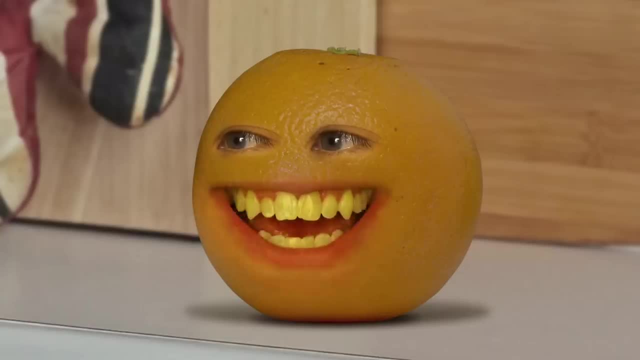 I have an HO. I have nothing, Not even hands. All right, Pear Orange is beating us. We gotta get Orange a letter. You guys couldn't get me a letter, even if you had a stamp. Don't worry, I have a great idea for a super difficult shot you'll never be able to make. Watch this. 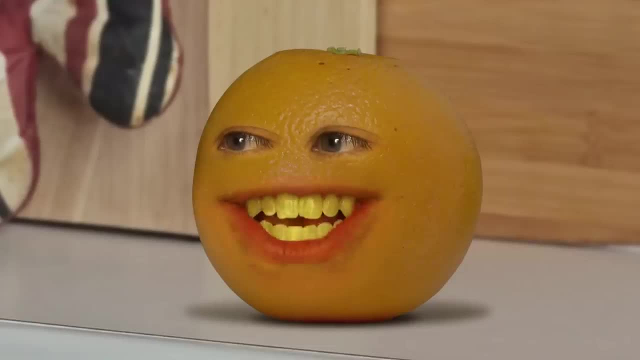 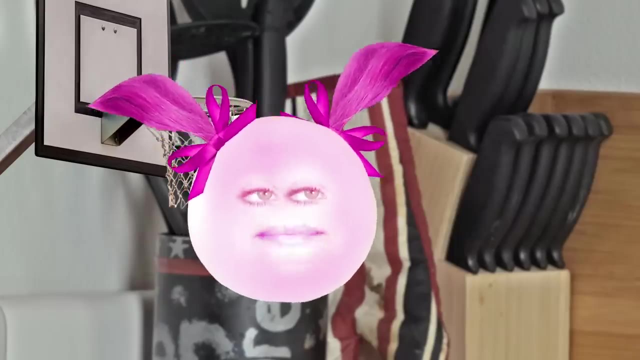 Huh, Hiya guys. Whoa, Who knew the neighbor kid was such an airhead? This isn't even as big as I can get. I can get way bigger if I have more gum, but my mom says I should eat my vegetables if I want to get bigger someday. 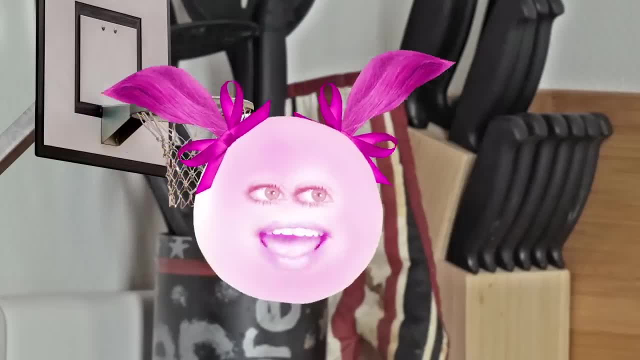 but that's gross because vegetables taste gross, And it also strikes me as a moral gray area because some of my best friends at my old kitchen were vegetables. I can't shoot. She's blocking the hoop, So bounce it off her, Okay.